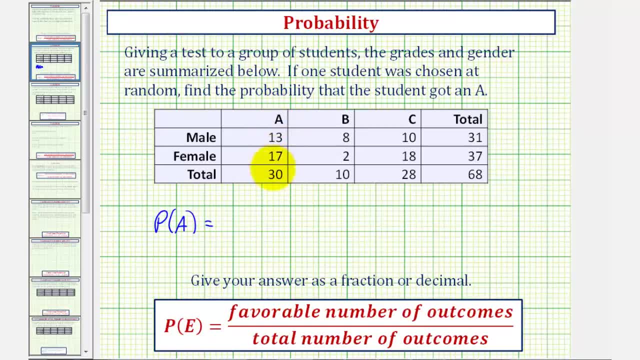 notice how this column here tells us the number of A students. There were a total of 30 A students, thirteen of which were male, seventeen of which were female And, looking at the totals column notice, thirty-one males took the test. thirty-seven females took the test. therefore there were a total of sixty-eight. 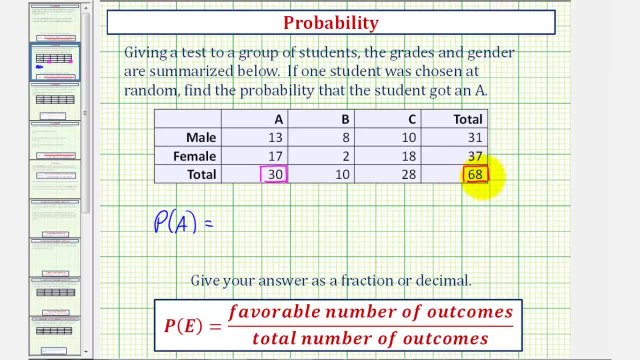 test takers. So of the sixty-eight test takers, thirty received A's, And therefore the probability that a student chosen at random would have gotten an A would be the number of students receiving an A, which is thirty, divided by the number of students that took the test. 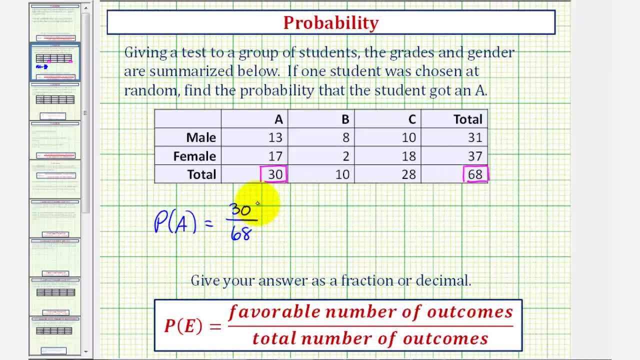 which is sixty-eight. So this is the probability. but we are asked to express the probability as a fraction or a decimal. If we do express it as a fraction, we do want to make sure the fraction is in simplified form. Notice: thirty and sixty-eight do share a common factor of two. 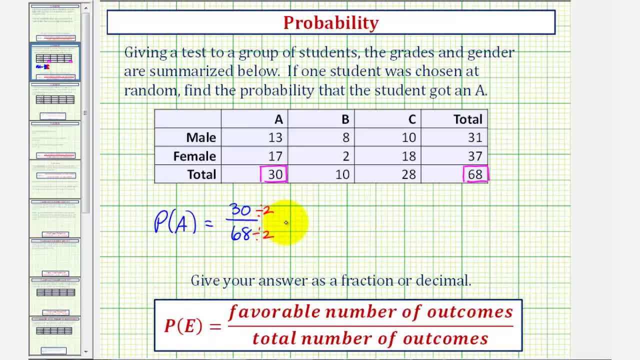 And therefore, as a fraction, the probability of an A would be fifteen thirty-fourths. This fraction is in simplified form. Let's also give the probability as a decimal and even though it doesn't ask, as a percentage. So to convert the 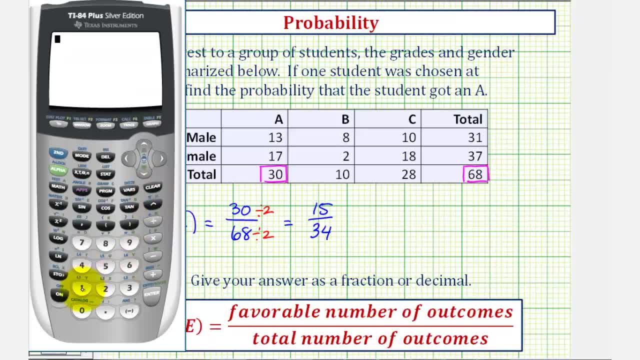 fraction to a decimal. we'll divide, So fifteen divided by thirty-four. Let's round this to four decimal places. So this would be approximately zero point four, four, one, two. Notice how the seven indicates to round up. So the decimal value is going to be an approximation. 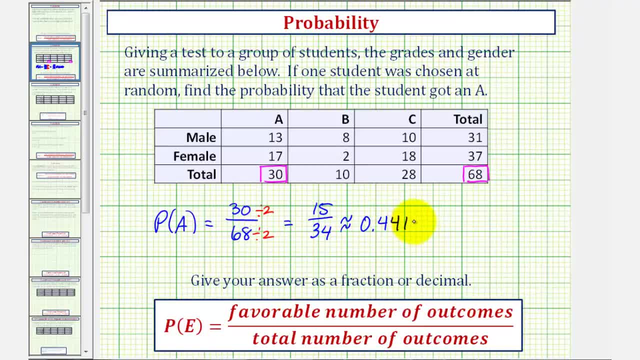 Zero point four, four one, two. Let's also write this as a percentage. To convert a decimal to a percentage, we multiply by one hundred and add a percent sign or move the decimal point to the right two times. So this would be forty-four point one two percent. But it is important to keep in mind. 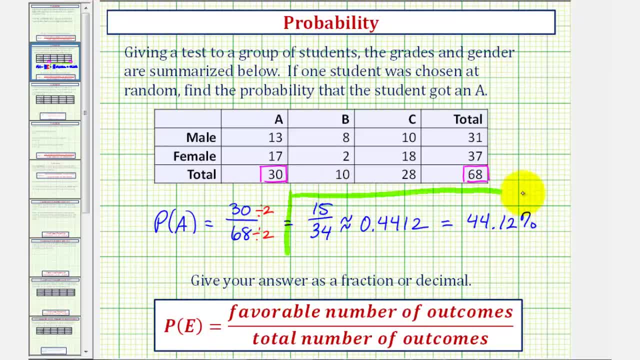 that the fraction is the exact probability of an A, And the decimal and percent are rounded approximations. I hope you found this helpful.